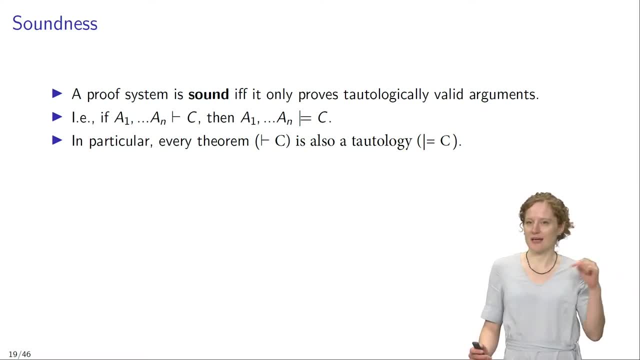 conclusion c: from premises a1 to an, then the argument from a1 to an to c is tautologically valid. We can also express this idea using our new symbols. So in a sound proof system, if a1 to an turnstile c, then a1 to an double turnstile c. Now, as a special case on this: 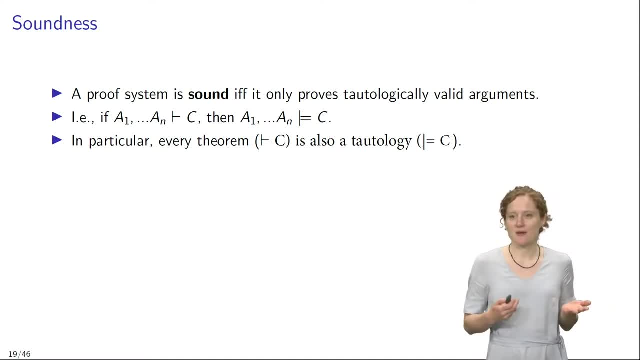 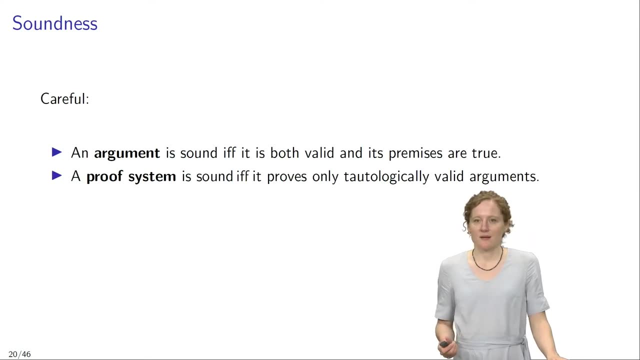 general property. In a sound proof system, every theorem is also a tautology. Now be careful, since we actually have used the word soundness before and had something very different in mind. So earlier in the course we said that an argument is sound if, and only if, it is both. 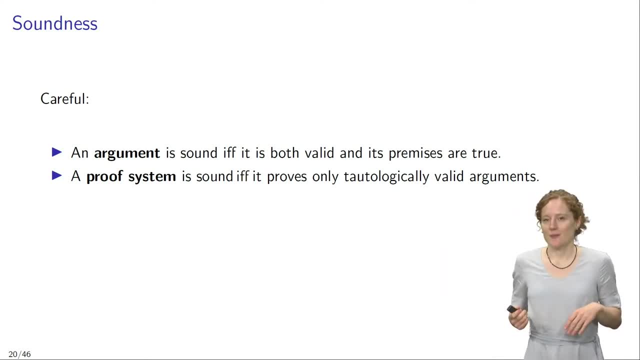 valid and its premises are true. But now we are talking about something very different. Now we are talking about properties of proof systems and we are saying that a proof system is sound if it proves only tautologically valid arguments. So whenever the word sound appears, try to reflect on the context and think about whether 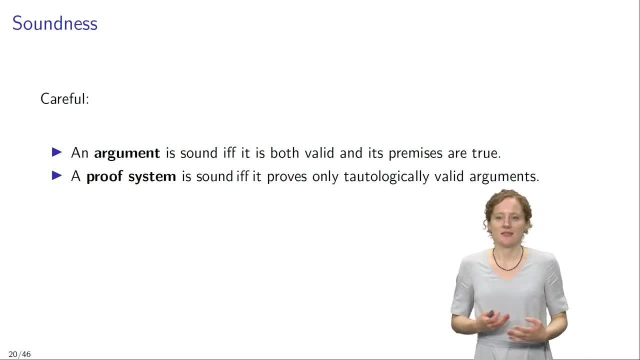 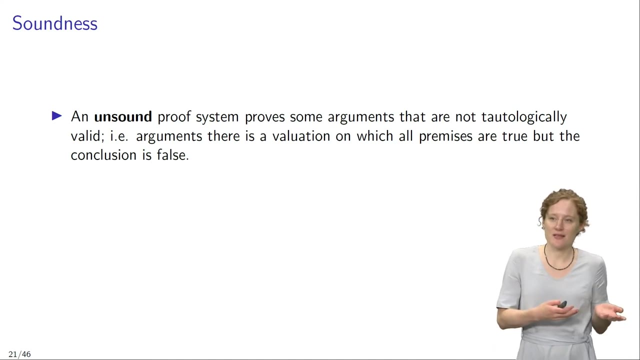 the author has arguments or proof systems in mind, since soundness as applied to arguments is something very different as soundness as applied to proof systems. Now, an unsound proof system proves some arguments that are not tautologically valid, meaning arguments for which there is a valuation on which all premises are true, but the conclusion. 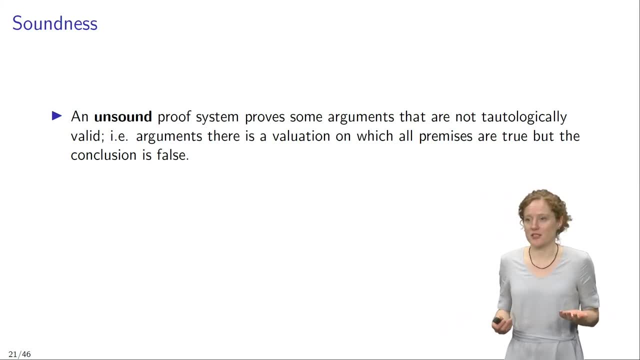 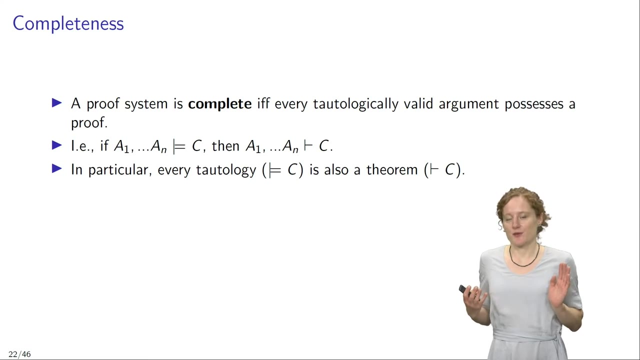 is false, And that's the bad making feature. We don't want a sound system, a proof system that would allow us to prove such bad arguments. The second important virtue of proof systems that we are going to discuss here is completeness. A proof system is complete if, and only if, every tautologically valid argument possesses: 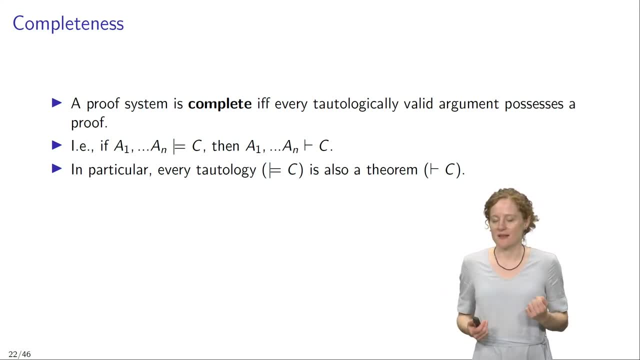 a proof, And so that means that whenever the argument from A1 to AN to conclusion C is tautologically valid, then we can also derive the conclusion C from premises A1 to AN, And we can express this property using our new symbols.